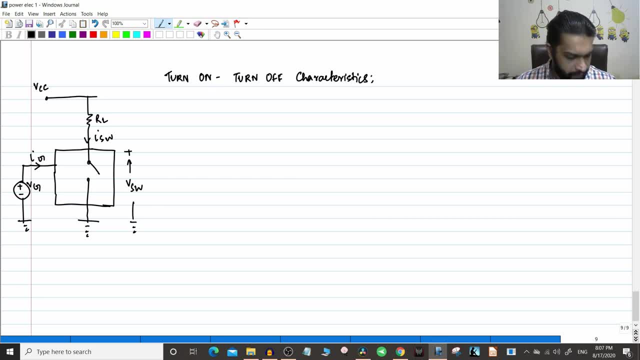 So what should be the turn on and turn off characteristics. So firstly here. the third point now will be the turn on, the turn on and the turn off process. and the turn off process should be what It should be: instantaneous. it should be instantaneous. The idea is that, for example, there is a switch. 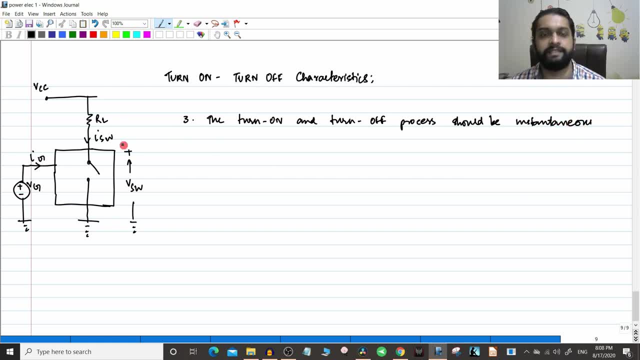 and you are turning the switch on. Okay, so, for example, let us take this case here Now, when the switch is off, okay, for example, the switch is off here, So this is an open circuit, right? So if you do a little bit of KCL here- sorry, KVL here- you will get. 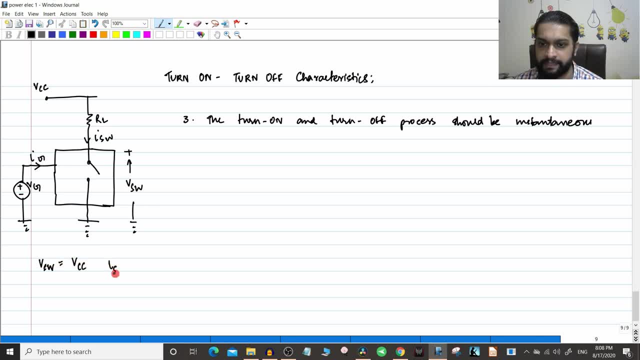 this switch voltage will be equal to VCC And this ISW will be equal to zero, because naturally the current is: this is turned off, Turned off right. This circuit is an open circuit, So ISW is equal to zero and this voltage 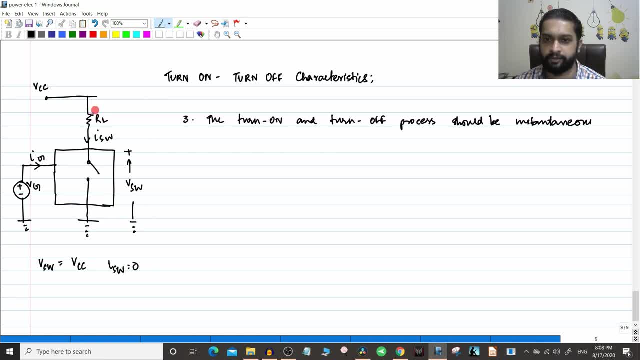 VSW will be equal to VCC. Okay, so that is the basic idea. There is no current drop here, So the VCC will be coming and VSW will be equal to simple KVL here. Now, when you are switching this on, for example, this is the condition when it switched on. this is like: 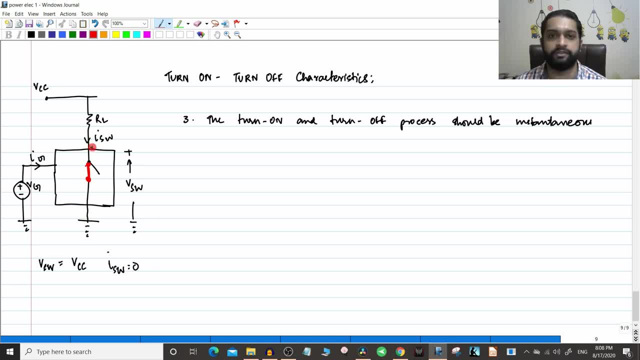 a free path, right, This R on is equal to zero, tending to zero. So in this case, when the device is on, so this is off condition and this is on condition. So VSW will be equal to zero, And whereas ISW will be equal to VCC divided by RL here, right The simple. 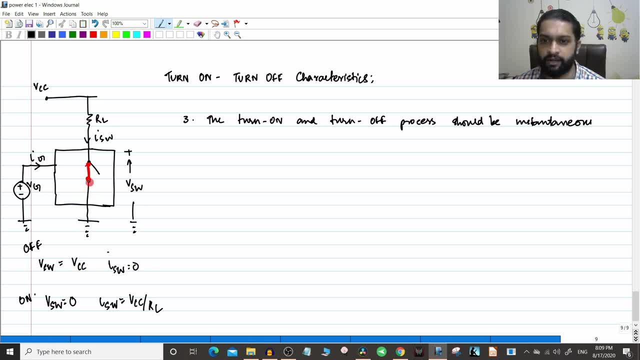 application of KVL and KCL. So when the switch is turned on- that is here you are, like having a short circuit path- the voltage across the switch will be equal to zero. that we have already seen. in an ideal case, right From the off state to the on state, the switch voltage goes from VCC to zero and the current 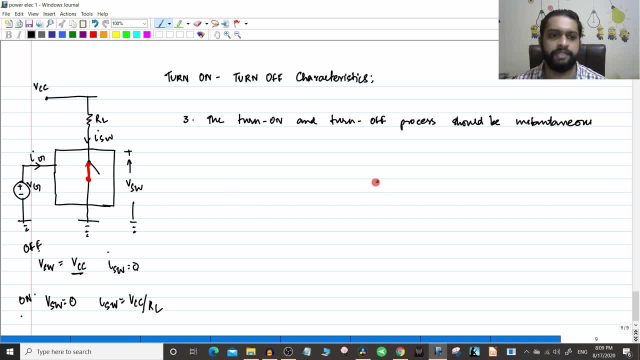 goes from zero to VCC divided by RL. So if you just want to plot it in a graph, okay. So for example, we can take: this is VSW and this is your ISW, So we will draw it for the ideal case. So, for example, it is getting turned on at this point here. This is with. 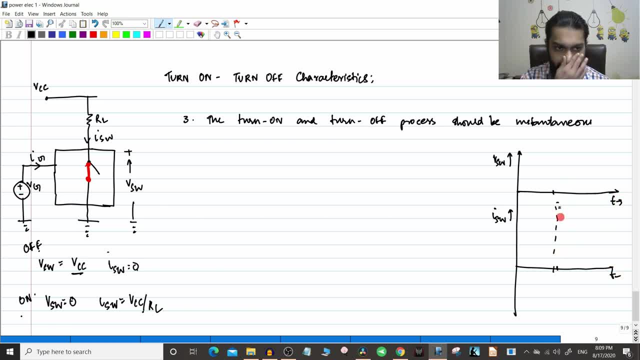 respect to time. Okay, so this is the point where the switch is going to turn on. So before it is turned on, it is turned off, right? So that case, VSW will be equal to VCC. VSW will be equal. 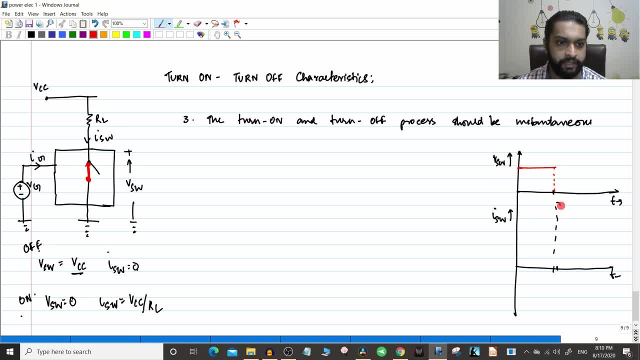 to VCC till the point where the switch is turned on. So at this point, switch is on. switch is on at this point and exactly at this point. So we will call it as say: T on, At T on point: the switch is on. 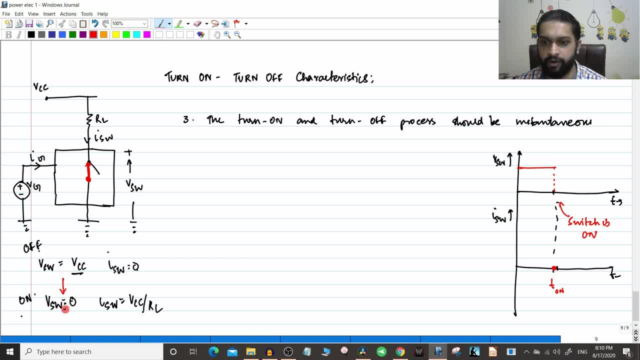 So at that point, what will happen to VSW? When the switch is on, VSW will become equal to zero and it will continue till the switch is turned off. okay, Whereas what happened to ISW? ISW initially it is zero, okay, Switch. 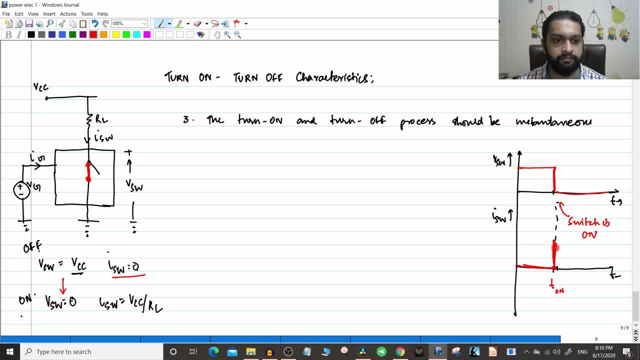 is off, it is zero. But when the switch is turned on, it will become this value, that is VCC divided by RL. So here switch is off and here switch is on. So these are all ideal characteristics. When we see the practical condition, you will see that it takes some specific amount of. 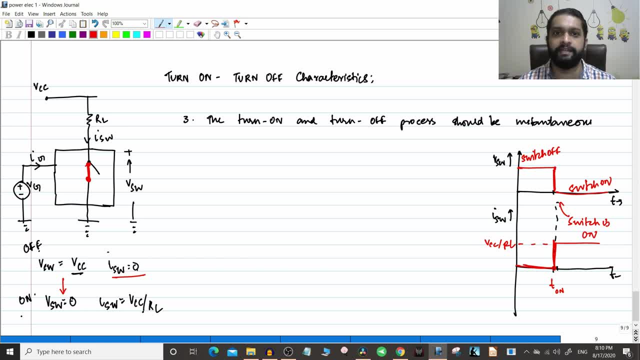 time before the switching action actually happens. okay, So there will be something which is called a rise time, delay time, storage time and all those things. okay, So that we will see when we are seeing the actual characteristics. So the basic idea is that the turn on and 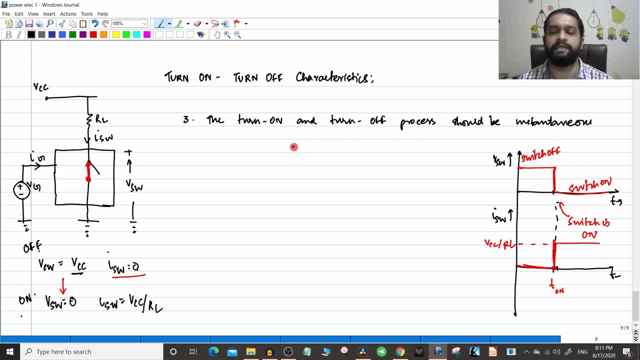 turn off process should be instantaneous, And so all the timings associated with that should be equal to zero. The switch should also be on. The switch should also be on. The switch should also be off. Open like this: Instantaneously it should close, or instantaneously the switch should. 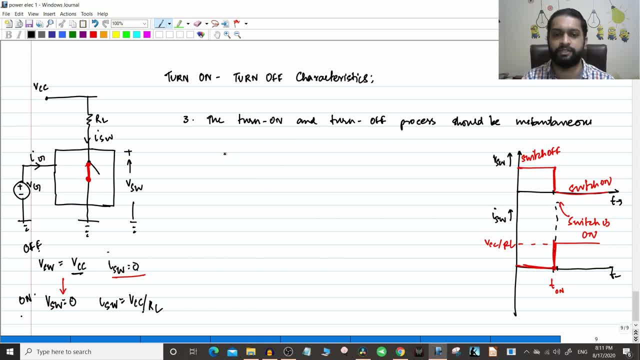 turn on. So there are some terms for the time being. just listen to those terms and when we see the practical graph we will understand it properly. So this is for the ideal switch. This is for the ideal switch, And so the first case a. 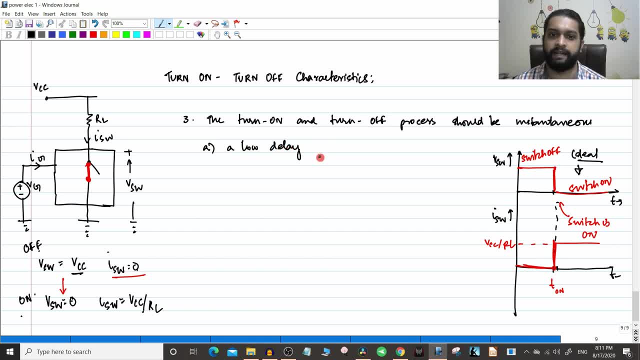 low delay time. These definitions we will see in the practical graph. The low delay time Td tending to zero. That means any delay, any delay in the turning of the switch should be equal to 0.. There are proper definitions for this that we will see in the next video. 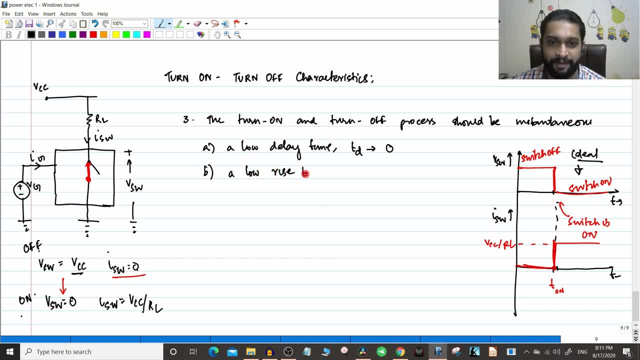 A low rise time. I am not at all comfortable without explaining, moving on like this, but unfortunately for this topic you have to wait. So rise time should be equal to 0 and then should be a low storage time, because in this characteristics the delay time, rise time. 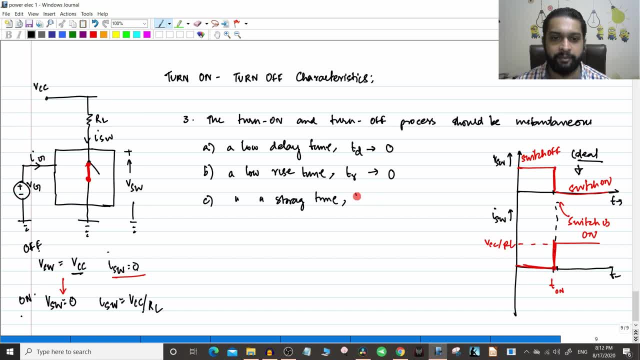 storage time are not there. How can I explain that? So, for example, just remember that there are certain times which we timing, values, which are defined, and all those should be equal to 0. Storage time should be equal to 0 and d- a low fault time. a low fault time. 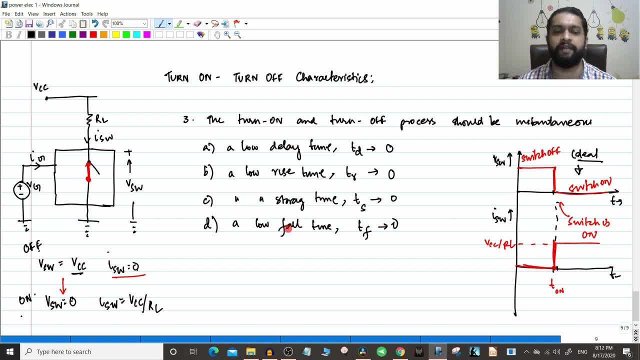 this tf tending to 0.. You can see that all these times have a name. clearly that is showing some kind of a delay on the operation of the switch. that is, from the turn off condition to turn on condition, You are having these two. This is from off to on. That is there is some delay to actually. 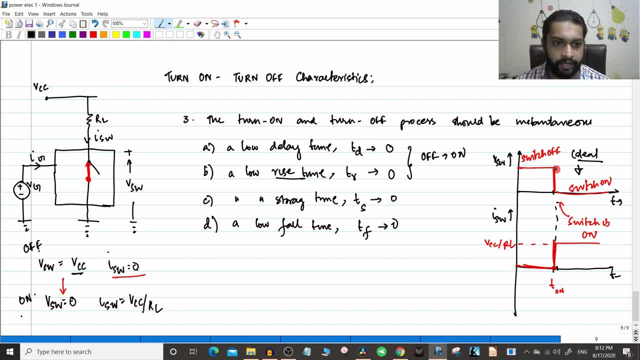 start the switching action and from this point, from off to on also, there is another delay time that is actually the rise time. So this is from off to on and this is from on to off, That is, once you turn off the switch, it will take some time for the action to start. the 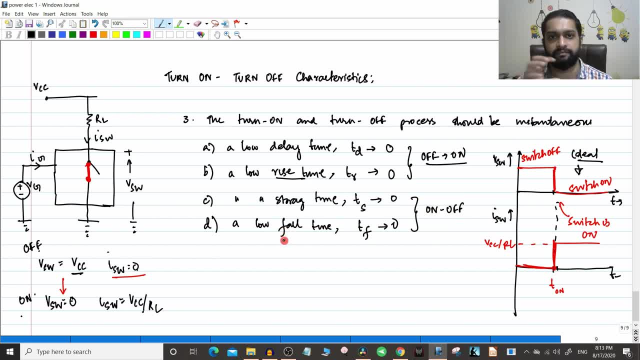 turning off action to start, and the turning off action, the total actual time that is taken, is also called the fault time. So this is off to on. So when we draw the actual graph for a practical switch, it will be more clear. Now the next thing: what do you require to turn on the switch or turn off the switch? 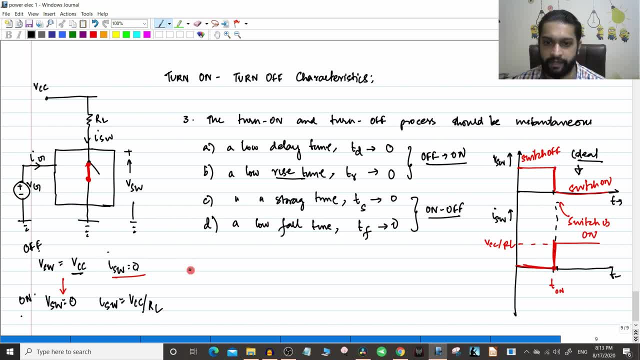 you require the gate pulse. So gate pulse is a very important component here. So the next point is regarding the gate pulses. So we will write the point here- for turning on, for turning on and turning off of the switch. This point is with regards to the gate power for turning on and turning off. it requires 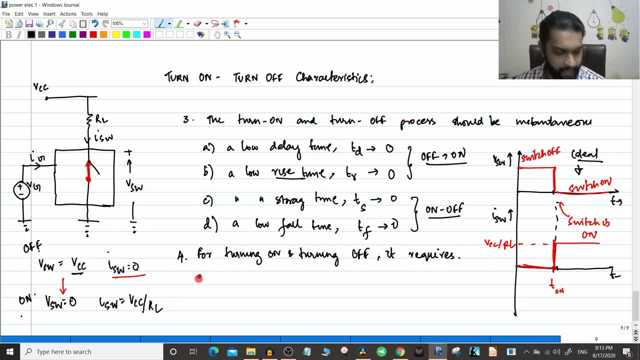 that is the ideal switch requires a very low gate power. Ideally, see, just like in a transformer, we assume that the excitation current is almost equal to zero. but it should produce flux. practically it is not possible. you should have some excitation current, So similarly here the gate power should be as minimum as possible. So for an ideal case, 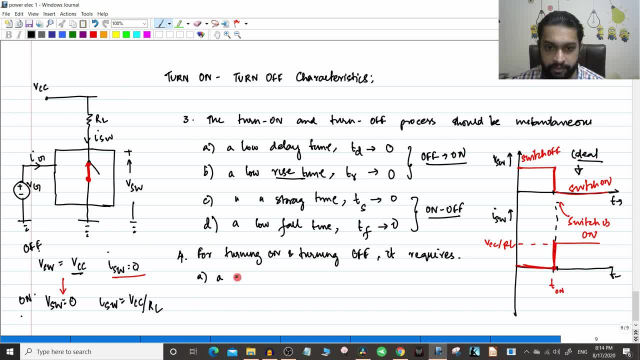 that will be tending to zero. Okay, So you need a low gate drive power, because the gate drive power is something which is actually driving the switch. it is not taking the actual current. So these all should be as minimum as possible. so to avoid any kind of losses, or like to. 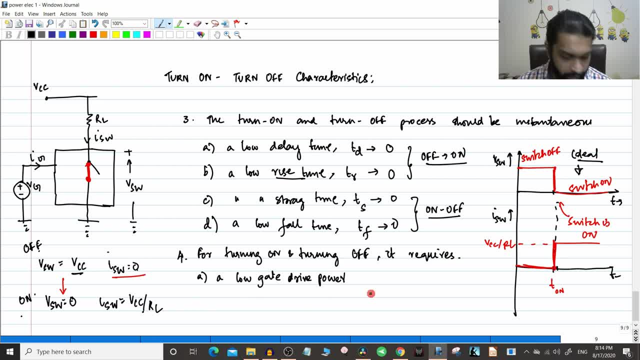 minimize electrical consumption of the switch as such. So it should have a low gate drive power pg and that is tending to zero b and for that what you need: a low gate voltage, A low gate voltage vg tending to zero. these are all simple terms I think you can understand. 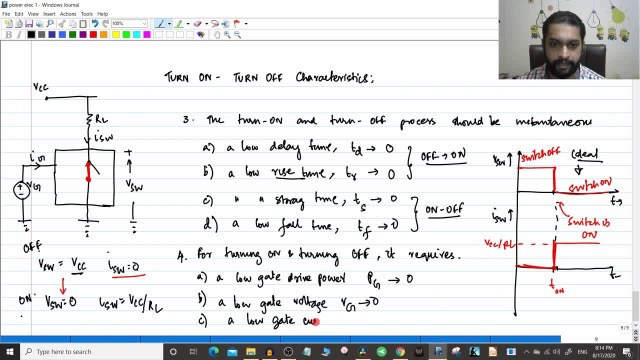 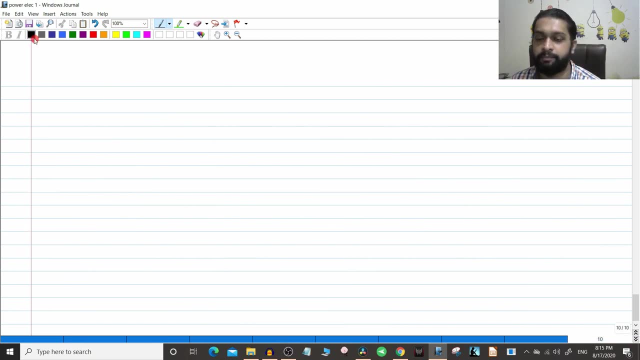 and a low gate current and a low gate current ig tending to zero. Therefore, the gate also will be- should be- a low gate power drive pg tending to zero for the ideal condition. Now the next point is that next point is also an important point, that is, the turn on of 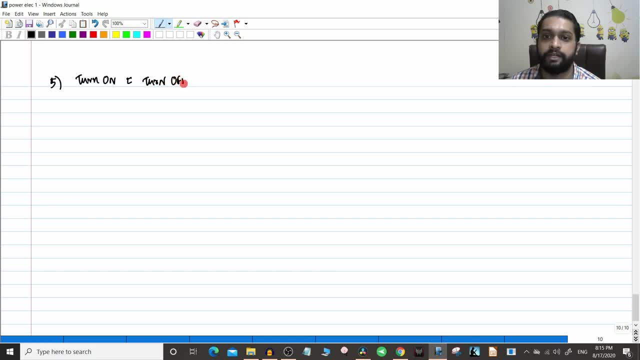 the switch and the turn off should be controllable. turn off should be controllable. That means you, based on your wish, you should be able to turn on or turn off the switch. Okay, So that is the basic idea. So what the ideal switch requires is that for turning on, you will have a gate pulse. 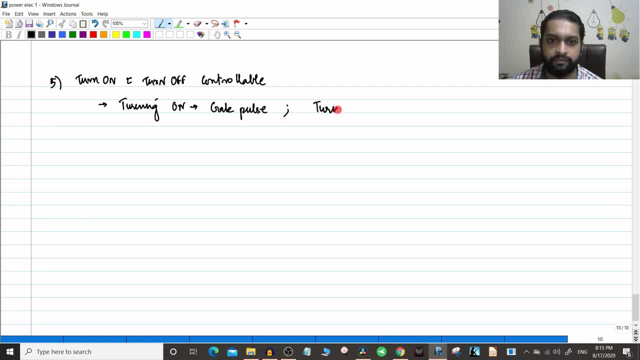 gate pulse and also for turning off you can have a gate pulse. So all these concepts, we will be going into more depth when we see the actual device, like an SCR or a triac and MOSFET etcetera, about how turning on can be done through a. 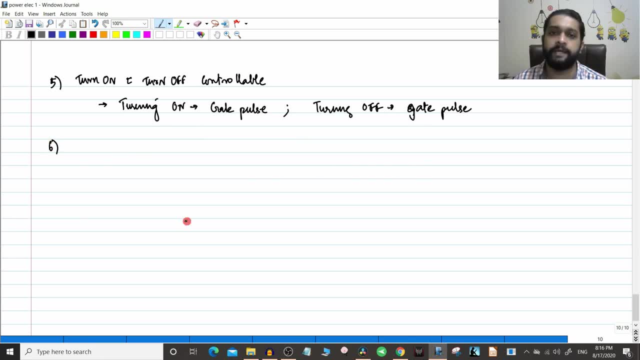 gate pulse and a turning off can be done through a gate pulse. Now we are just going through the broad characteristics. So turn off and turn off should be controllable for a switch, for a good switch. Next one: the turning on, the turning on and the off condition. 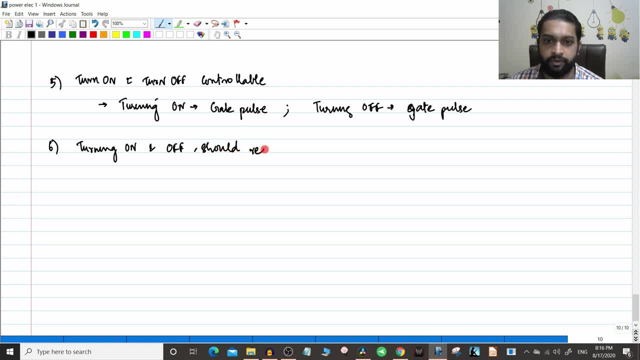 Okay, So turning off should only require a gate pulse. should only require a gate pulse. That means the signal that you are using to turn on should not be a continuous signal. That means the value of ig should not be something like: if you are turning on at this point should. 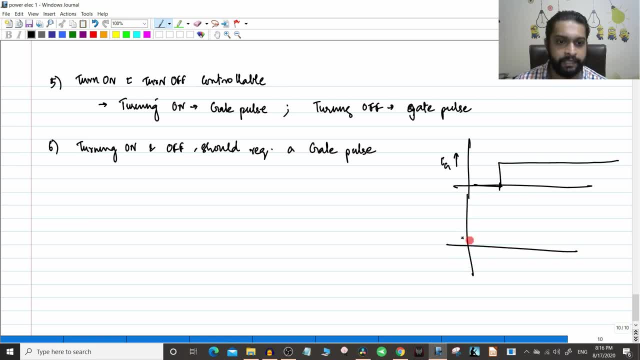 not be continuously going like this. The device should be turned on just by using a pulse, like this. This should only be sufficient to turn on the device. It should not be like this. It should be turned on using a pulse and turned off using a pulse. 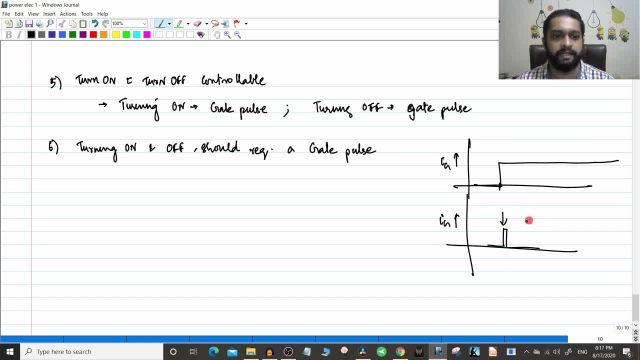 You can clearly see, because the ig value is small pulse, The average value of ig will be very low and therefore the pg, that is, the gate drive, also will be very low. So the turning on and turning off should only require a gate pulse, okay. 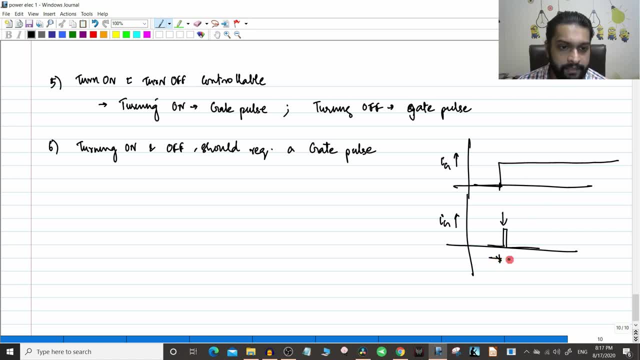 And gate pulse. so if you call this as pulse width here, This width of this pulse you call as pulse width and that width is tw, because this is with respect to the pulse width, With respect to time. that is the pulse width. the pulse width tw should be tending to 0.. 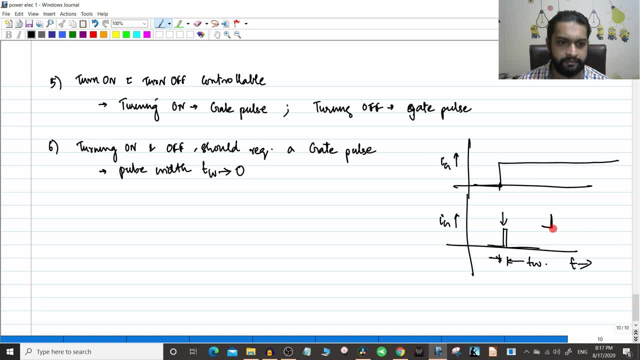 That means it should be a very, very small pulse. okay, like this, something like this: okay, So that is the ideal. characteristic means that pulse width should be tending to 0.. Next point is that. so the major points are over, and next point is the dyb dv by dt rating. 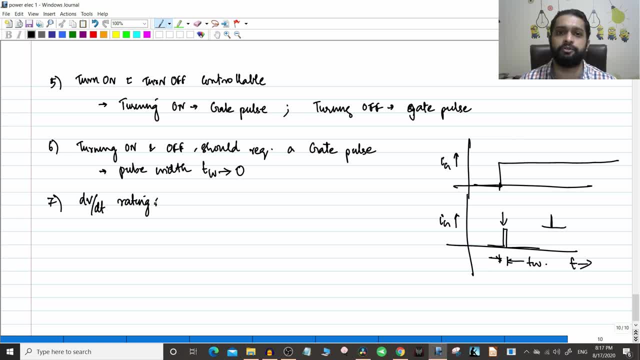 So in some cases you might have that the device might be subjected to huge amount of voltage fluctuations. That means the dv by dt rating, dv by dt- might be very high, So the device should be able to withstand that okay. Therefore, the dv by dt rating, dv by dt rating- should be tending to infinity. 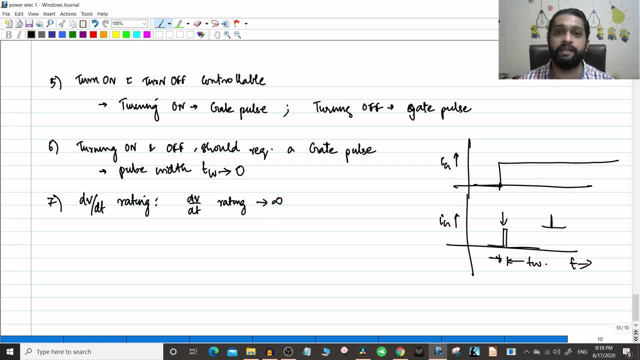 Why? to handle all observed or every high voltage fluctuations? okay, So that is the basic idea. So why it should be tending to infinity. to handle rapid changes in the pulse. So that is the basic idea. So why it should be tending to infinity. 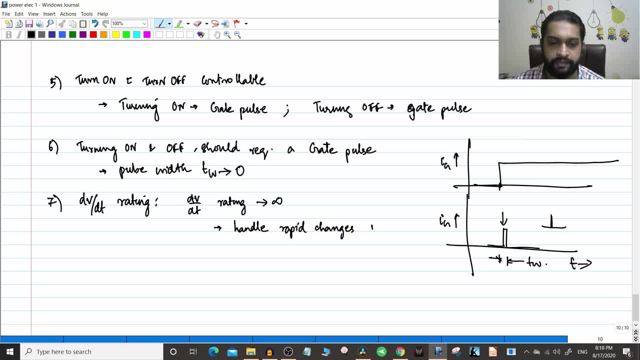 To handle rapid changes in the pulse. So when somebody is designing a switch they will try to make dv by dt as high as possible. Next is di by dt rating. You know that in certain cases there can be a huge rate of change of current right. 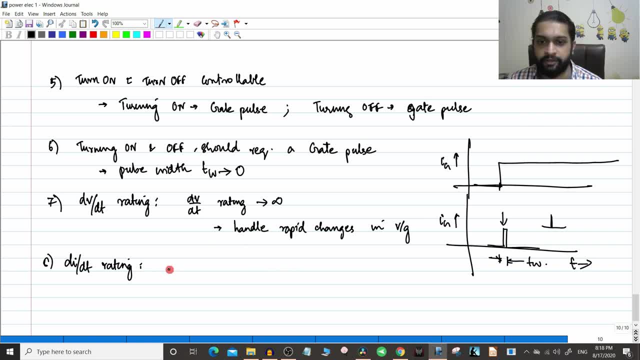 In some devices they have huge rate of change of current, So in that case also the switch may be damaged. but your switch should be able to withstand all those things. Therefore the di by dt rating also should be tending to infinity. Why to handle? to handle rapid changes in current. rapid changes in current, okay. 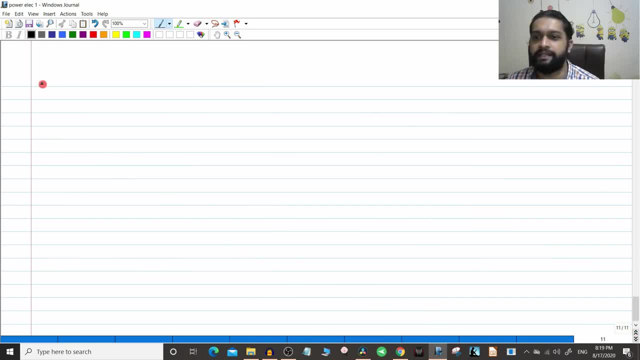 So that is another thing And you know that any device, any switch or any device in generally will heat, right, If it keeps that heat within itself, it will burn. It has to transmit it to the atmosphere that the heat should move from the body to the. 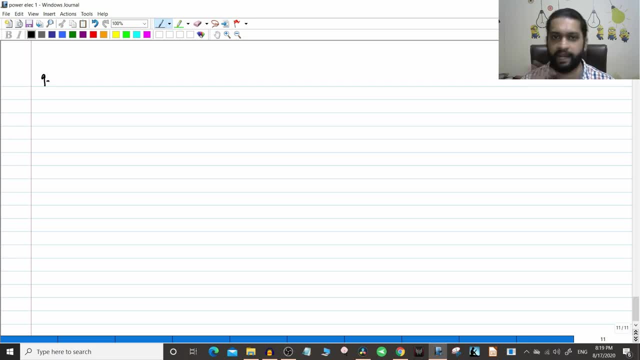 atmosphere. So that process should happen Very easily in an ideal switch. So it should be able to transmit the heat. Transmit the heat to the ambient, to the ambient easily, Transmit heat to the ambient easily. So there is a technical term for this, that is this called thermal impedance. 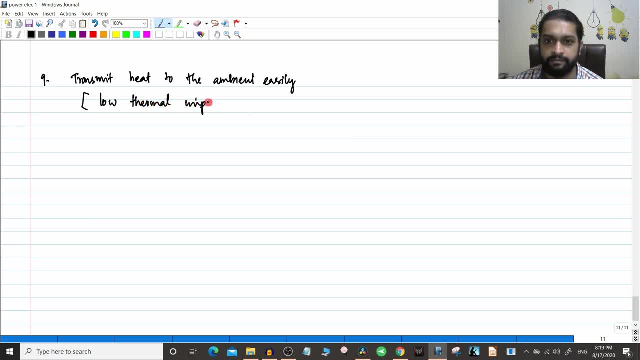 So thermal impedance should be low so that heat is easily transmitted from the device to the ambient. So the low thermal impedance from the, from the internal junction, from the internal junction to the ambient, So that is the basic idea. So this should be very, very low so that heat transmission is easy. 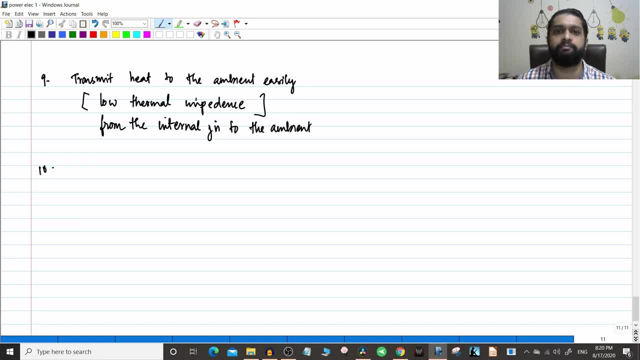 Next point. for example, sometimes the switch might be subjected to some fault condition. For example, you will have a simple switch, something like this, And there is a load. Okay, For example, this load takes 100 amperes in normal condition. You are saying 100 amperes in normal condition. 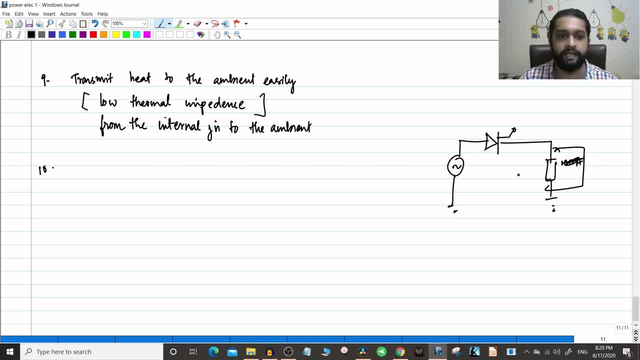 Sometimes what happens? it might have a short circuit. A huge amount of current will be going And that current is not normal current. 100 amperes was the normal current. Now, whatever current is flowing is called the fault current In power systems and all you might have studied fault current analysis and all. 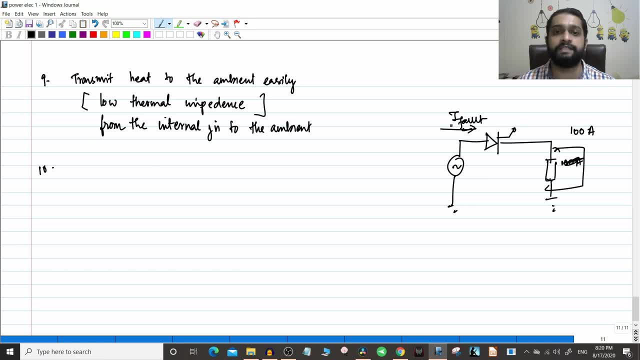 So this fault current should be the ability to withstand. this fault current should be there with the switch. Okay, So what we write here is that it should be able to sustain. it should be able to sustain any fault current. That is the ideal switch. we are always talking about the ideal. practically it will not be. 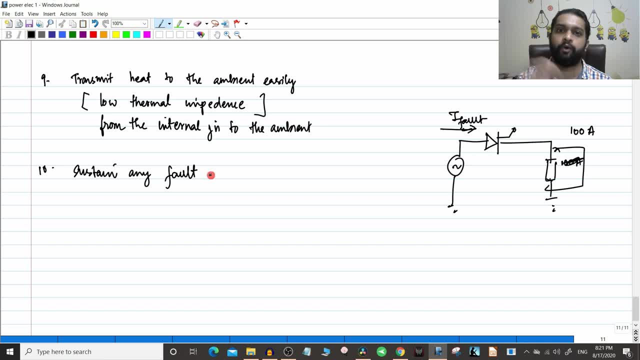 possible and the manufacturer will give you a specific value over which the fault current cannot happen. Okay, But for ideal switch, it should be able to sustain any fault current, any fault current, for a long time, for a long time. See a lot of devices. 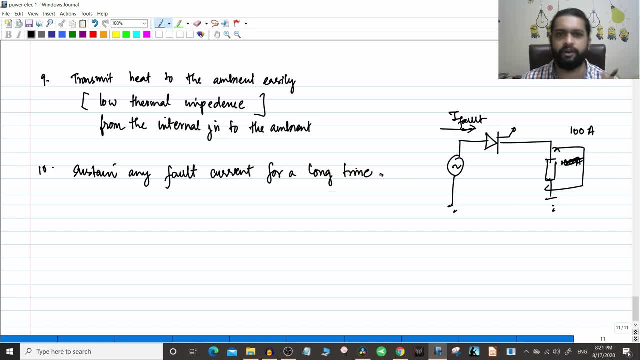 You see, they will be able to sustain any fault current. Okay, So it should be able to handle fault current for a short amount of for one second or for some milliseconds It might be able to handle it, not once again. So millisecond it might be able to handle, but for an ideal switch it should be able. 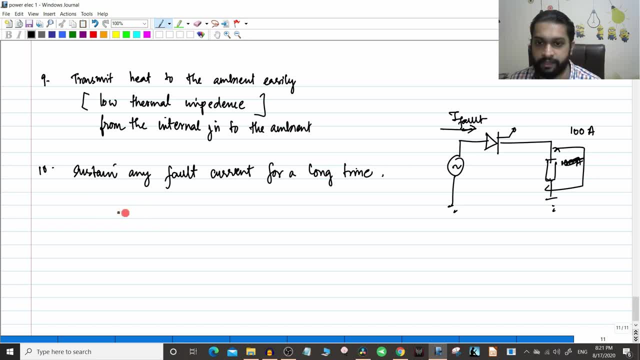 to handle it for a long time. That means, due to the fault current, there will be an I square T heat right heat. It should be able to withstand that heat and not be damaged due to that. So what we will tell is that the high I square RT rating right high I square RT rating tending. 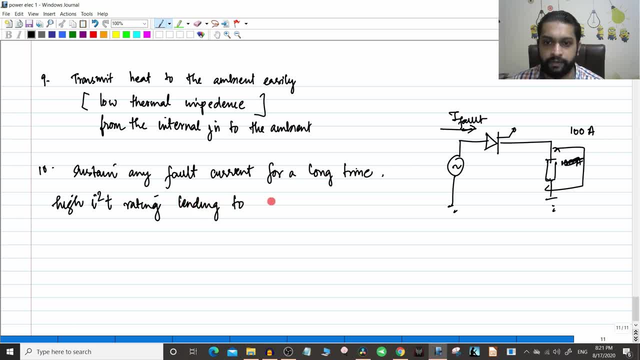 to infinity. tending to infinity because it is able to sustain fault current for a long time. ideal switch will have high I square RT rating. tending to infinity. that means for a fault current, which is for a long time, also the switch, nothing will happen for an ideal. 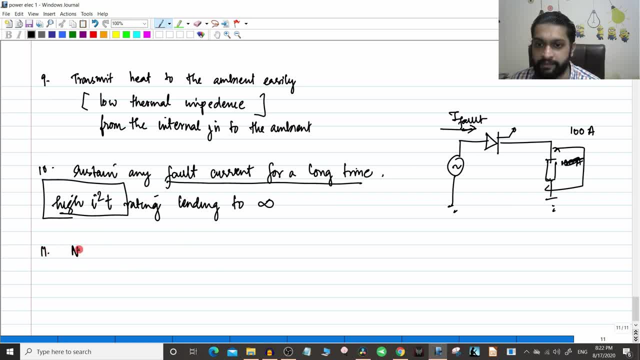 switch: Okay. Next one is the negative temperature coefficient of resistance. negative temperature coefficient of resistance: Okay, Basically, you know that in a simple resistance you are having positive temperature coefficient, that is, when the temperature increases, the resistance increases. So in this case, what will happen in the circuit in which that resistance is connected? the current will drop this. you do not want right. For example, you are having multiple devices connected like this in parallel. okay, multiple devices like this are connected in parallel to supply to a load, right, supply to a load. Now you are increasing this load current. Now you are increasing the load current. 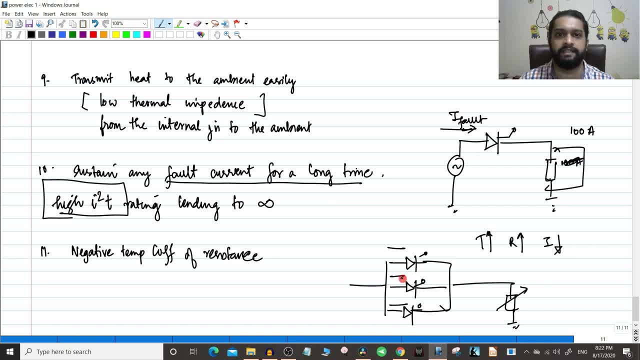 So through every device the current will start increasing. naturally there will be more heating it as compared to say, for example, T1 is at T1, is the temperature at T1 instant of time and you are increasing the load current right. So, for example, I1, T1 and we will call this as temperature 1. okay, I1 temperature and T1. 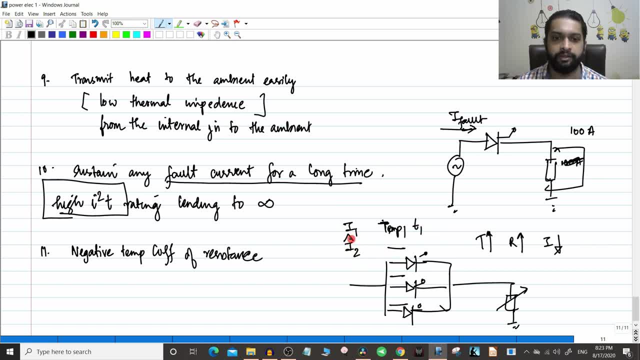 is for the first condition. For example, you increase it to I2.. Where I2 is the first condition, I2 is greater than you increase it to I2 and I2 is greater than I1. I2 is greater than I1.. So what will happen? T2 will be greater than T1, okay, and so what will happen? more heating. 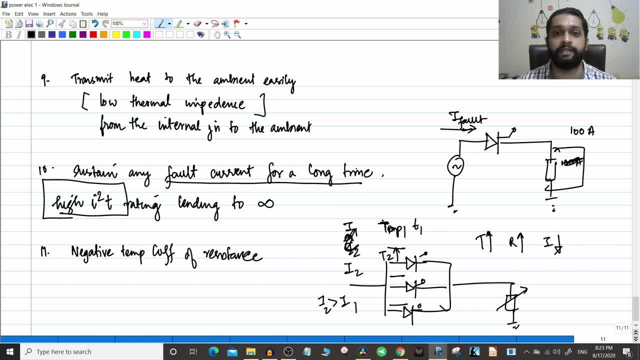 is happening Now. in this case, if it had temp positive temperature coefficient, this resistance will increase. this resistance will increase. So what will happen? some other device will get overloaded. So this device has my is getting overloaded, So that is not a good condition. 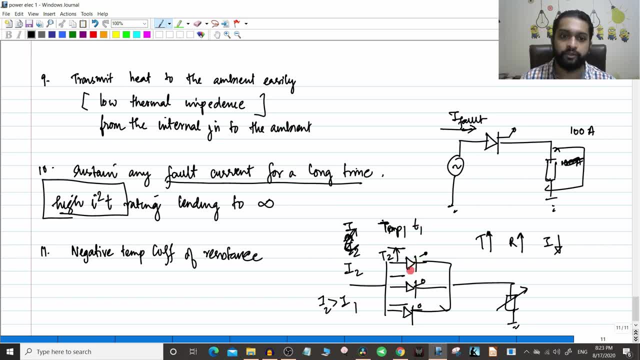 So as the temperature increases, its resistance should drop. Resistance should drop So that the current value is maintained properly throughout the circuit. So this is very important for current sharing. okay, So remember that there is no positive temperature coefficient. you should always have negative temperature coefficient. 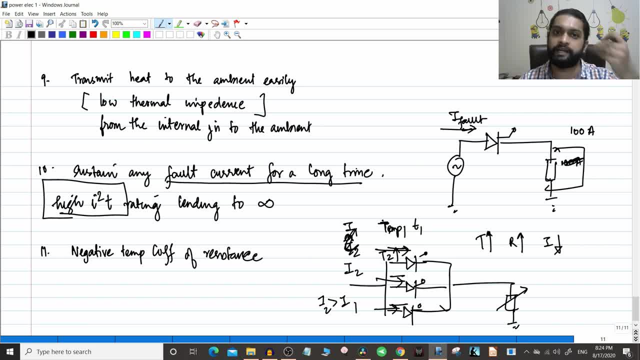 So that you can maintain proper current while you are doing current sharing. okay, So that is the point here. So negative temperature coefficient of resistance to maintain, to maintain equal current, equal current. Okay, So equal current sharing, equal current sharing when devices are operating in parallel, like 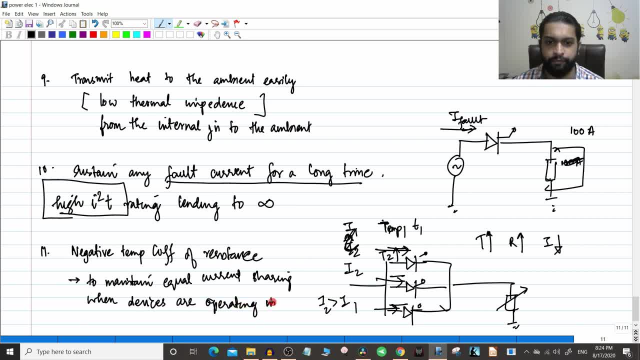 this operating in parallel. If it had positive temperature coefficient, what will happen? everything will have. the resistance will start increasing and the current will start dropping and all those problems will happen. But you do not want that. you are trying to increase the load current, So the device also should support that increase in load current, not oppose that increase in. 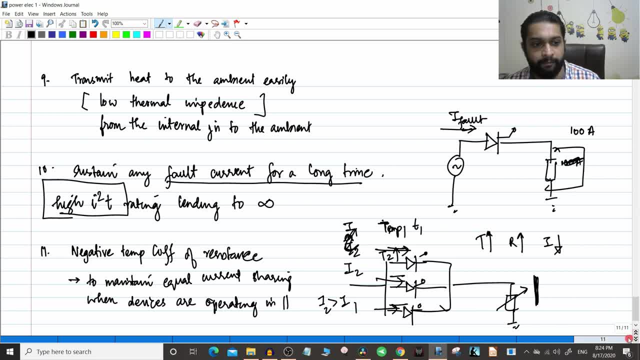 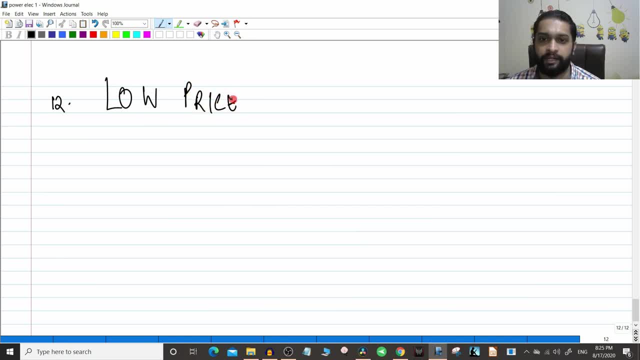 load current Right. So that is the basic idea. And finally, the most important criteria for the industry is that these switches should have low price. This is a very important criteria when you are talking about industries, that is, it should be of low price so that the industries can afford the switches. okay. 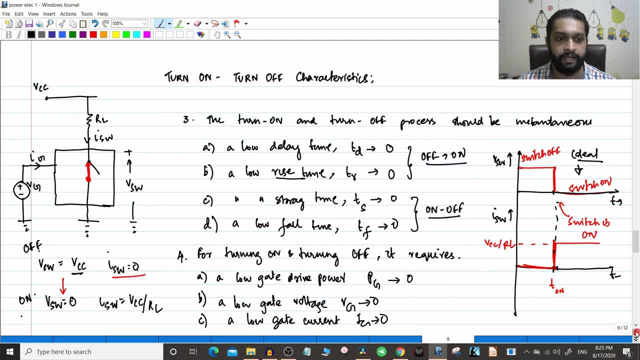 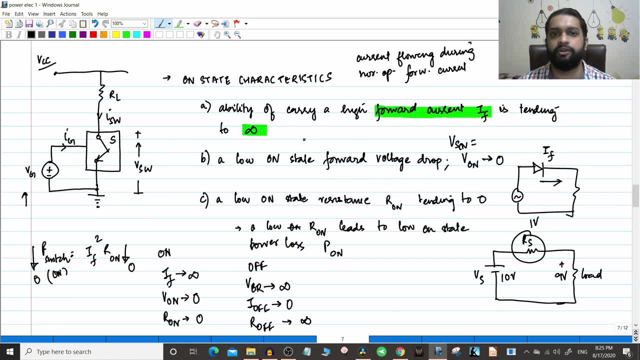 So we have seen a lot of points, So we will just go through them in a very fast manner. okay, So we started with the on state characteristics, right? So in on state characteristics, what do you need? You need high forward current, that is, if should tend to infinity, and the on state resistance. 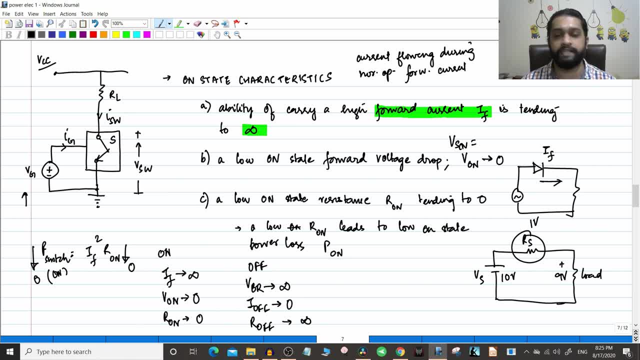 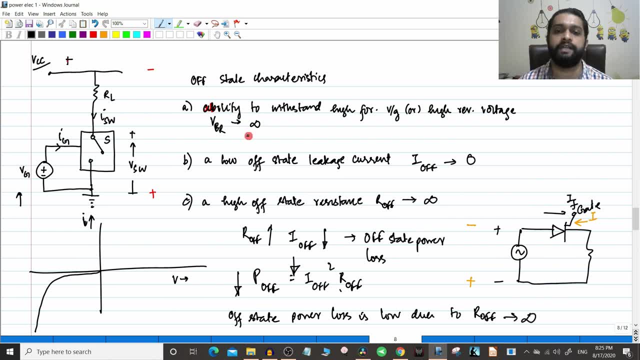 how. what should do? it should tend to zero and the on state voltage drop should also be equal to zero. So that is what we have seen in the previous video. Next for off state: in the off state, what I told you: when the device is in the off state. 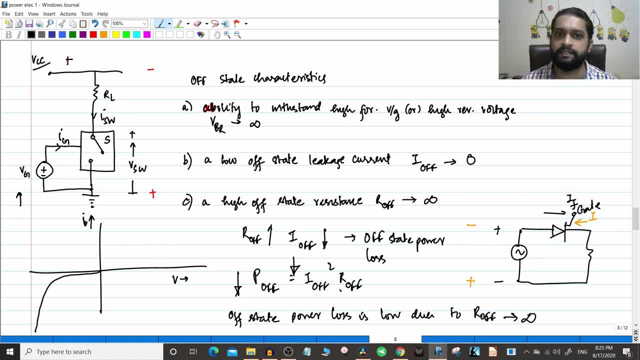 if you apply high voltage in the forward direction or the reverse direction, the it should not turn off. That means the ability to withstand high volt forward voltage or high reverse voltage. So that is what we have seen in the previous video. Okay, There is VBR should be infinity. 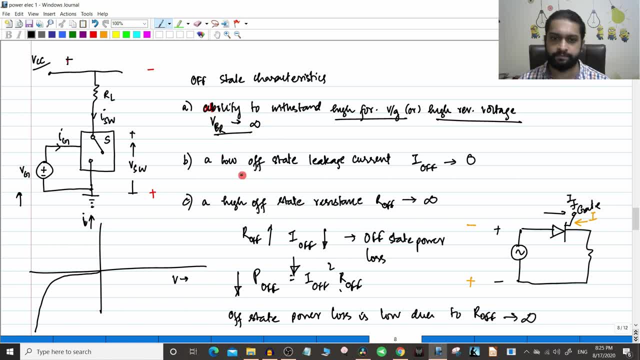 This is actually breakdown. VBR should tend to infinity. Then leakage current. I told you, all devices will have leakage current. for an ideal case, therefore, that switch should have a leakage current tending to zero, Whatever the off state resistance, because the device is turned off. 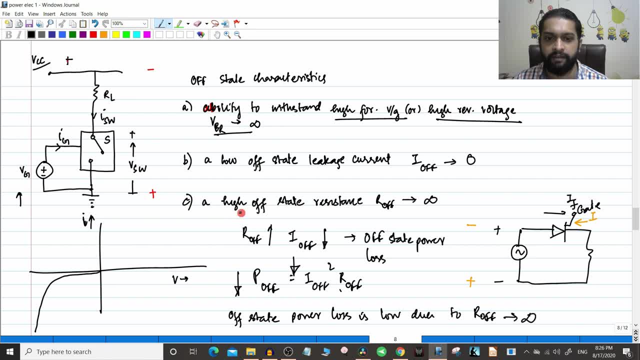 It means that it should provide very high resistance, right. So it should have high off state resistance, tending to infinity Also. the off state also, you should have low power loss. So this is the up state resistance, And in ON state also, the power loss associated with the switch should be tending to 0.. 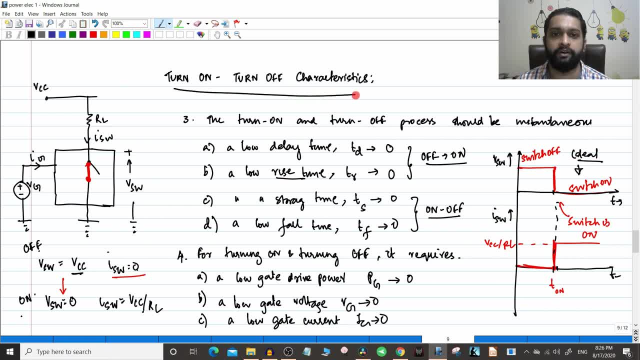 That is P ON, P OFF. both should be 0.. In today's video we saw turn on and turn off characteristics. I told you the turn on and turn off process should be instantaneous. That means all these current values, delay time, rise time, sorry time values, storage time, fault time- all should tend to 0. 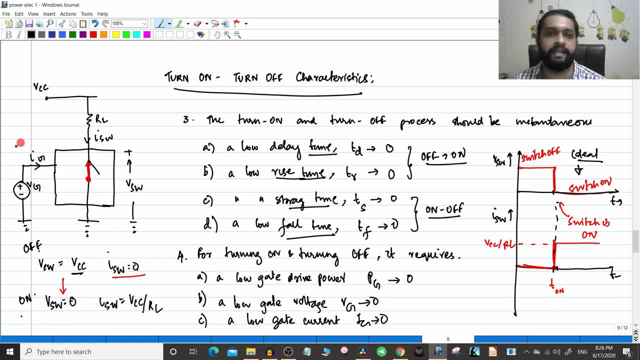 Then the gate drive which is used. this is the gate drive which is used That should consume minimum amount of power. Therefore, the PG gate drive power should be tending to 0.. For that, VG should be 0 and IG should tend to 0.. 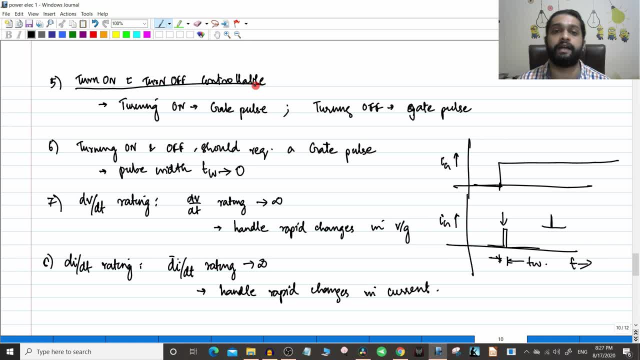 Then we saw that the turn on and turn off should be controllable. That is device should be able to switch on and switch off using a gate pulse. So whenever you want the device to turn on, you should be able to do it. Whenever you want it should be turn off, you should be able to do it. 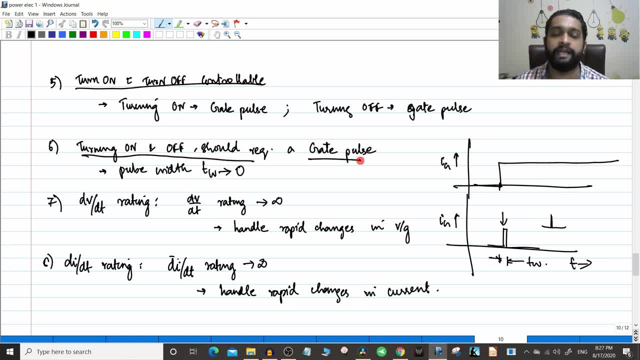 Then we saw that the turn on and turn off Should require only a gate pulse, not a continuous signal like this. It should turn on with a gate pulse like this, And this is the width of the gate pulse TW. That TW should be as small as possible so that it is a very thin pulse TW tending to 0.. 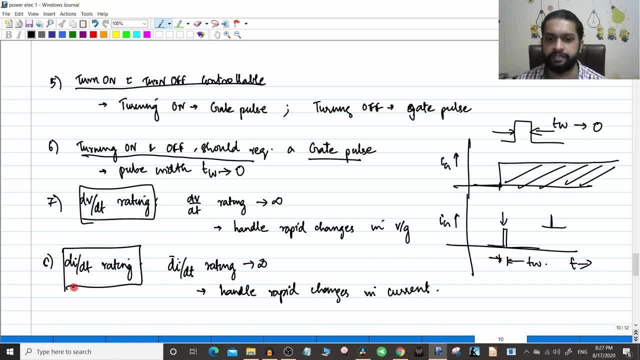 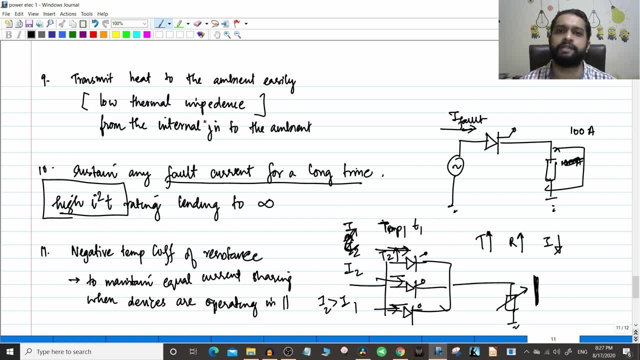 Then we saw the DV by DT rating should be high. DI by DT rating should be high to accommodate rapid changes in voltage and current. Then we saw it should be able to transmit heat to the ambient very easily, Otherwise it will get damaged. 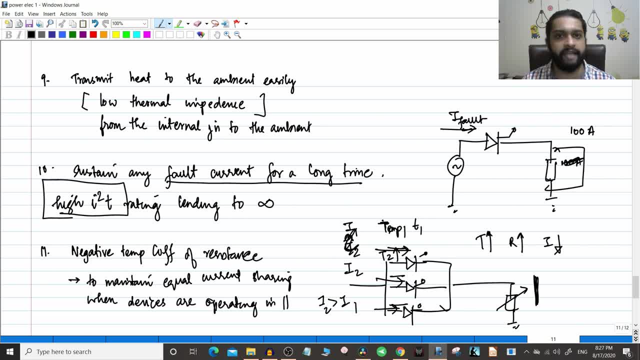 If every heat is localized in some area, it will get damaged over time. So an ideal switch should be able to sustain huge fault currents for a long period of time. So that is important: Huge fault currents for a longer period of time.